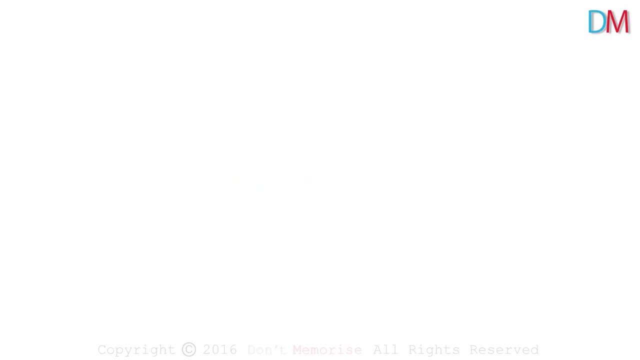 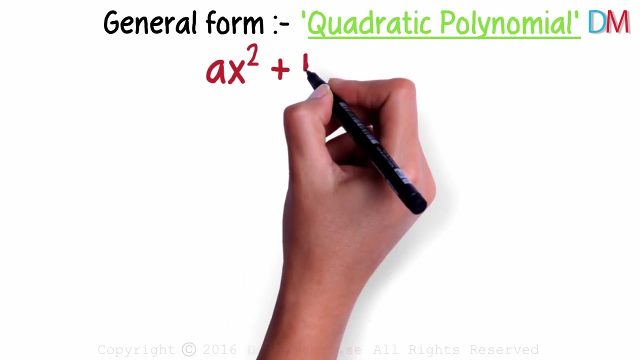 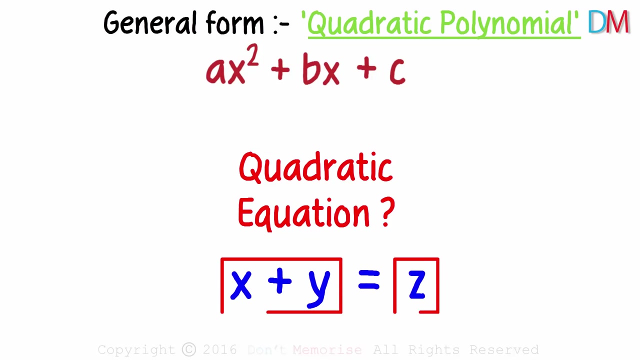 All of us remember what quadratic polynomials are. The general form of a quadratic polynomial is ax squared plus bx plus c. where the constant a is not equal to zero, The degree of the quadratic polynomial is two. So what's a quadratic equation? An equation, as we know, always has two sides. 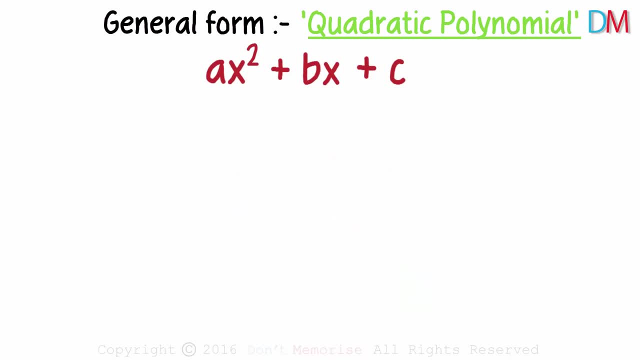 One on each side of the equal to sign. When we equate this general form of a quadratic polynomial to zero, we get the general or standard form of a quadratic equation. Remember that a is not equal to zero and the constants a, b and c are real numbers. 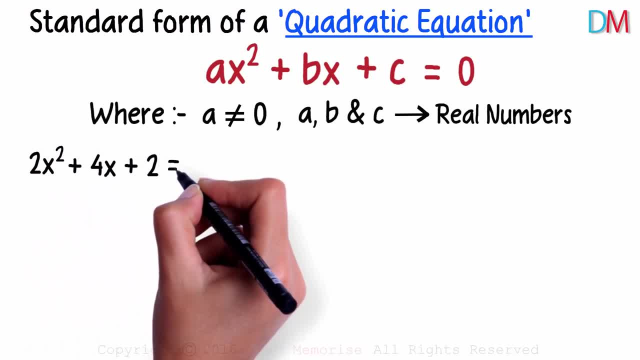 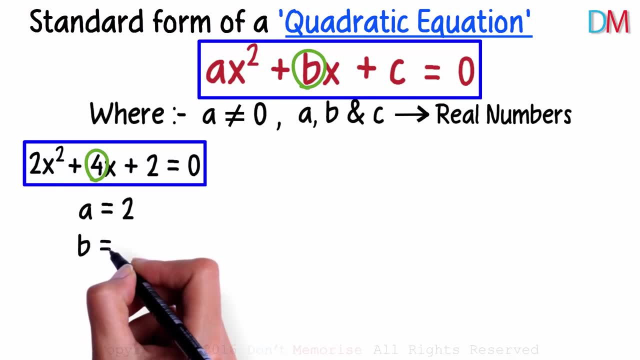 For instance, 2x squared plus 4x plus 2 equals zero, is a quadratic equation. Comparing it to the standard form, we get a as 2, b as 4 and c as 2.. a is the coefficient of x squared, b is the coefficient of x and c is the constant. 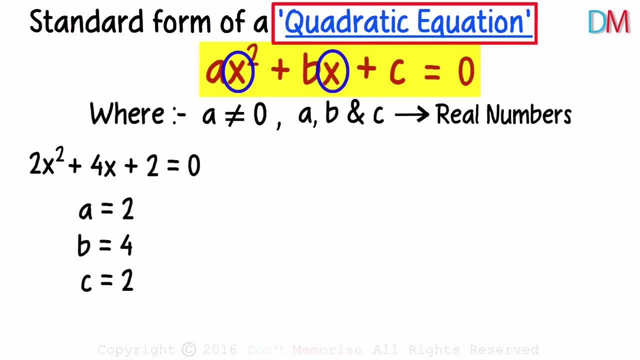 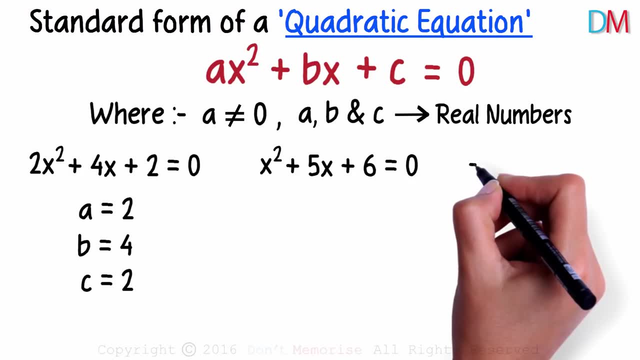 This is called a quadratic equation. in variable x, X squared plus 5x plus 6 equals zero, is also a quadratic equation, Negative: 3x squared plus 12 equals zero two. Yes, you might not see the x with power one in this equation, but it still is a quadratic. 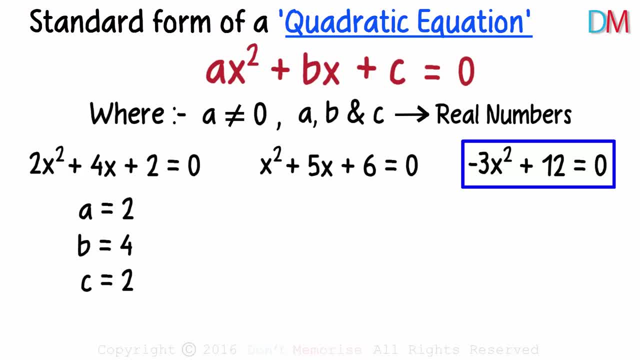 equation. That's because the degree of the polynomial is zero. The polynomial on the left is still two. Can you find the values of a, b and c in each of these cases? Here are the values. Notice that in the second case the value of coefficient of x is zero. 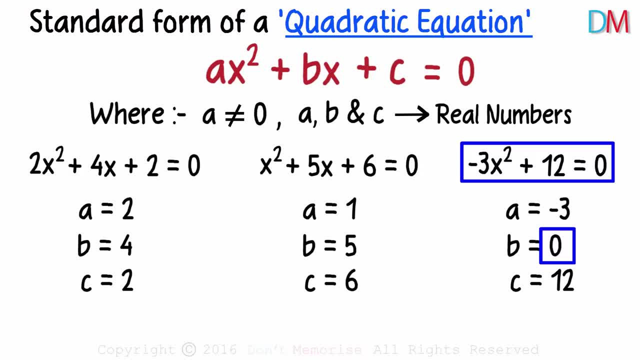 And that's not a problem at all. The important condition is that a must not be equal to zero. We can say that a coefficient of x is equal to zero, And that's not a problem at all. The important condition is that a must not be equal to zero. 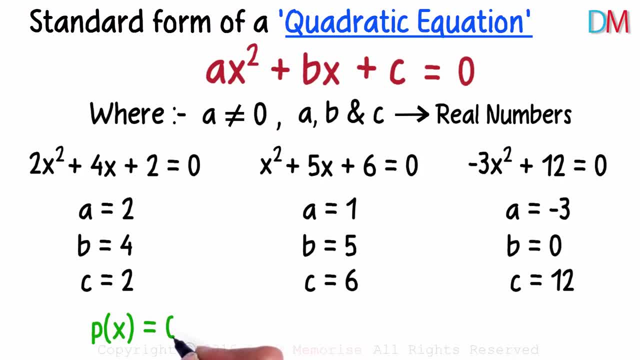 The important condition is that a must not be equal to zero. The important condition is that a must not be equal to zero, And that's not a problem at all. So the quadratic equation is of the form: p of x equals zero, where p of x is a polynomial. 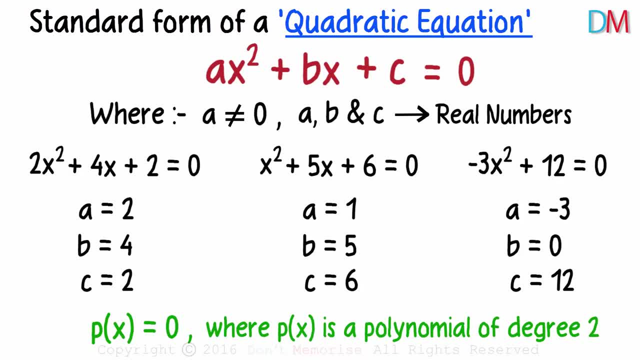 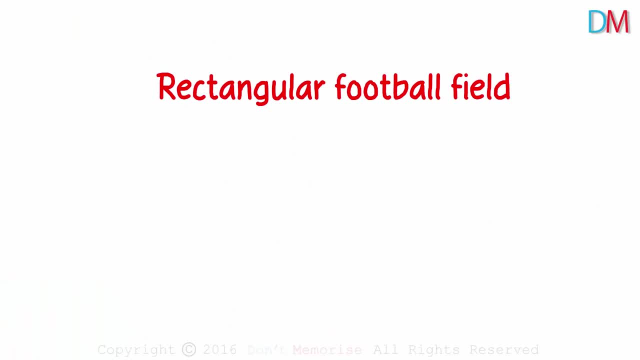 of degree two. Does it have any application in real life? Say, you are asked to build a rectangular football field with an area equal to 7000 square meters And you are also told that the length of the field should be 30 meters more than its width.